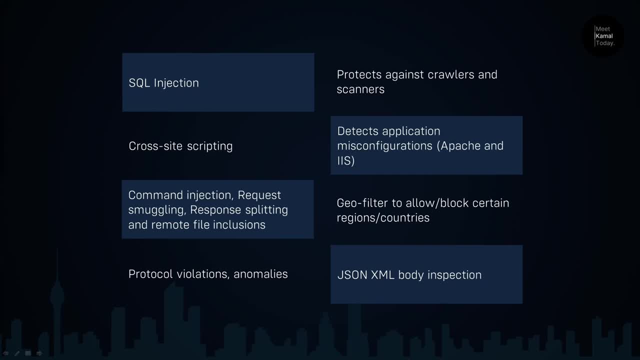 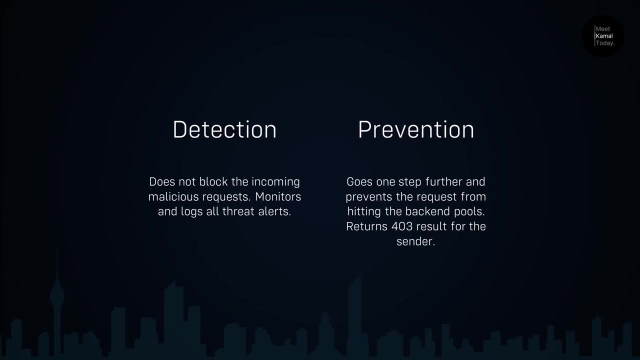 And I'm planning to do in another video on custom policies. And when you configure this, you have two options. You can configure this for detection or prevention. When you enable detection, web application firewall does not block the malicious request. It just log the information and metrics about the request and it will allow the malicious request to reach. 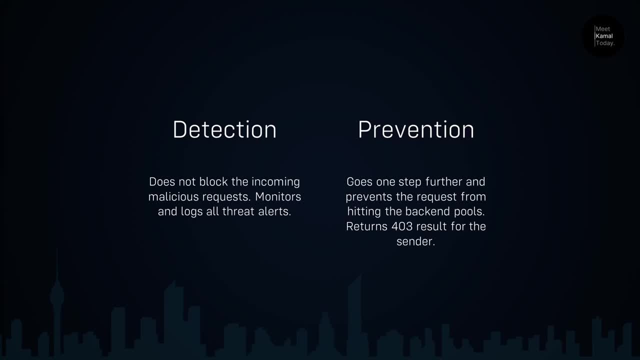 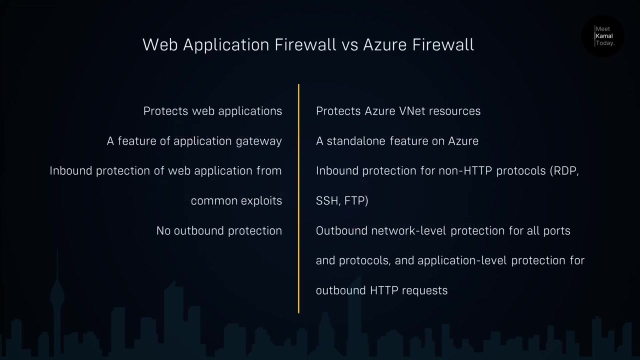 your backends. but when you enable prevention, web application firewall will block the request and it will return 403 http response to the sender or the malicious user. i'm sure you have heard about web application firewall and azure firewall as well. now let's understand the differences between these two services. web application firewall protects. 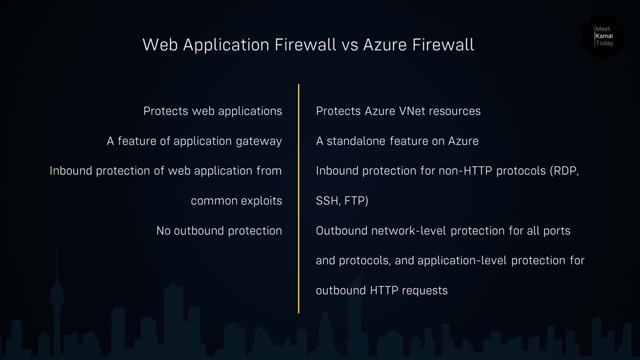 web applications and azure firewall protects as your v-net resources, and web application firewall is a feature of another azure service. it could be application gateway or it could be as your front door, as your firewall is a standalone feature on azure, since web application firewall is built for. 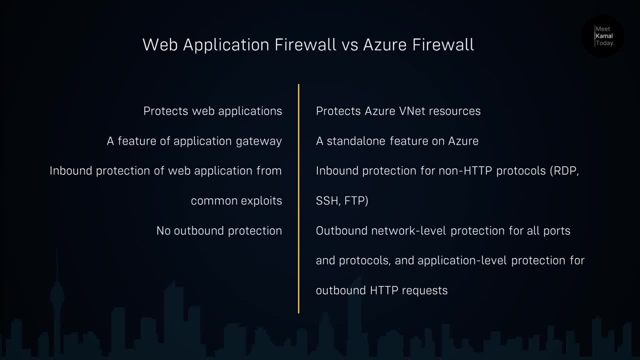 web request. it supports HTTP or layer 7 protection. azure firewall can provide inbound protection for non-data root power and access to your application's network from the end of the day for our client, but we need to understand the difference between these two services and with their applications. 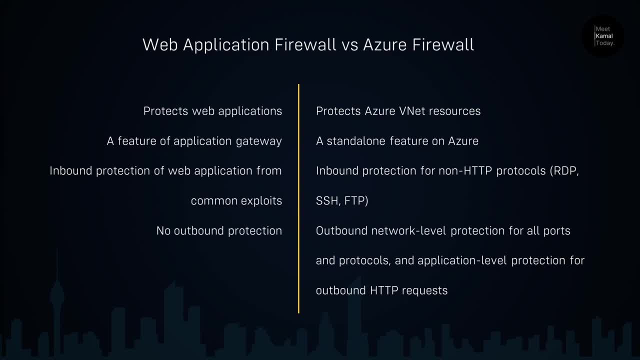 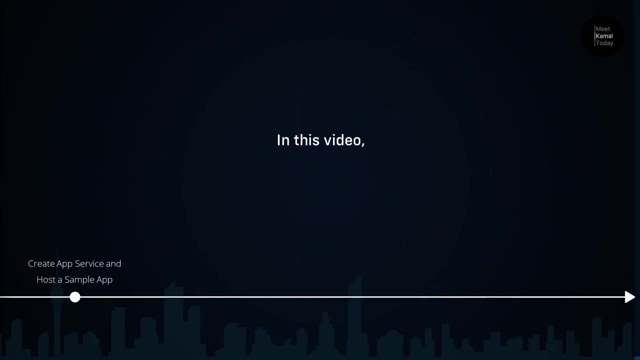 HTTP protocol, such as RDP, SSH and FTP as well, and also web application firewall, does not provide outbound protection, but Azure firewall has outbound protection features as well, and in this video I'm going to create an Azure app service and then I'm going to host a sample application. then I'm going to create an. 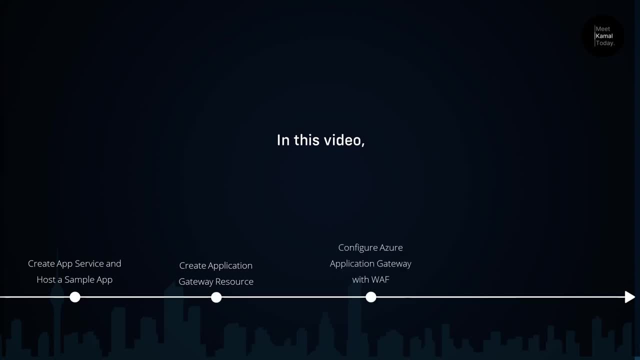 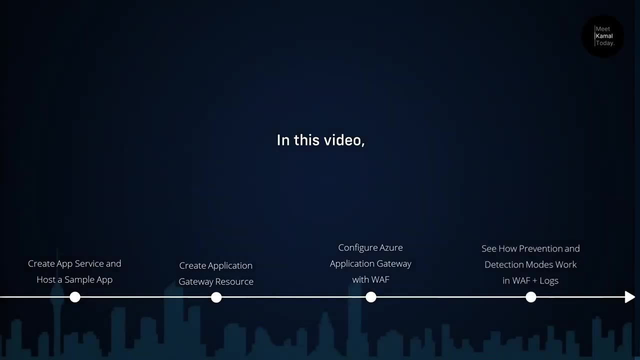 application gateway resource with web application firewall features on. and finally, I'm going to show you how detection and prevention modes work in WAF. I'm going to show you how to enable monitoring with log analytic workspaces as well. so let's get started. the first thing that I'm going to do is 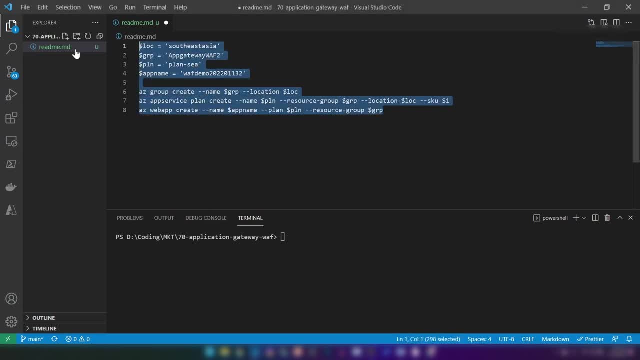 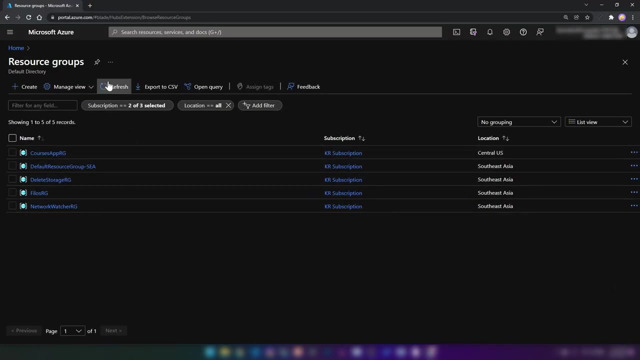 I'm going to create an app service for that. I'm going to run this script on my Azure PowerShell. let me do that now. all right, as you can see, our app service is in place. now I'm going into Azure portal and then I'm going to refresh it, and then I'm going to refresh. 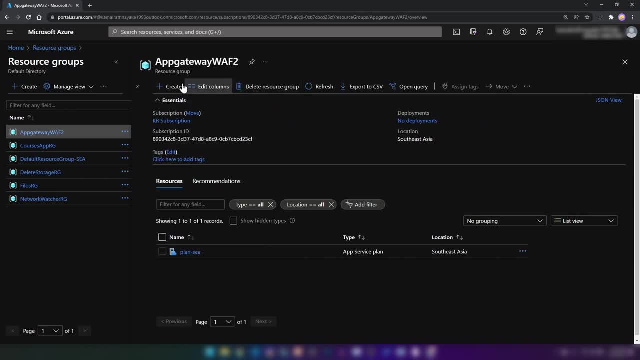 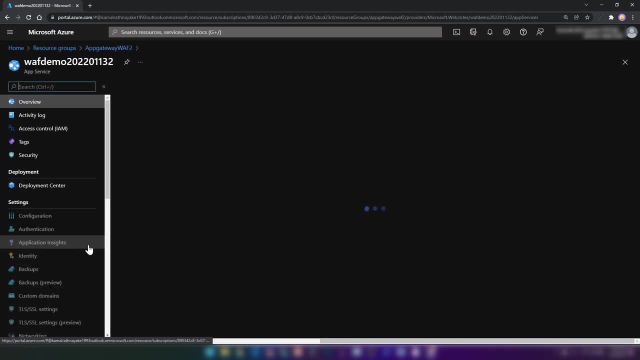 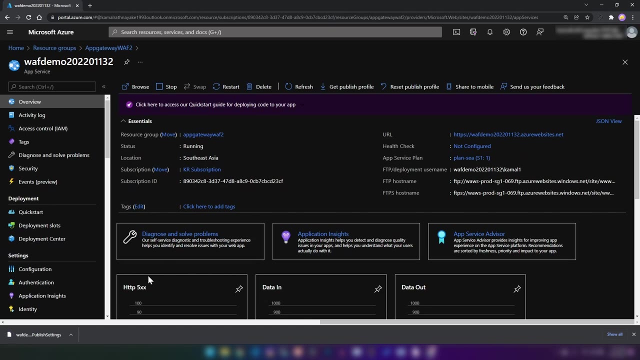 the resource groups. I'm going into the resource group that I have just created and let me click refresh again. as you can see, we have the app service here. now I'm going to download the published profile so that I can publish a sample application that will help us with our learning. now I have downloaded the published profile. 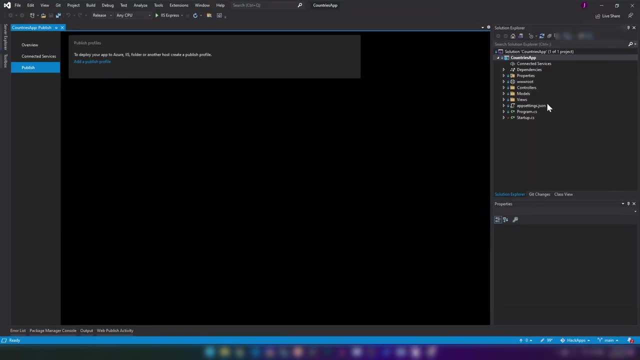 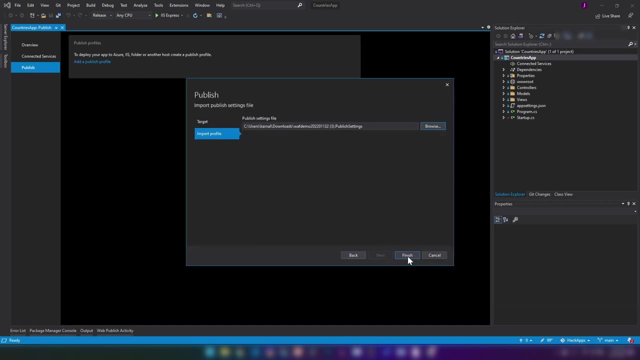 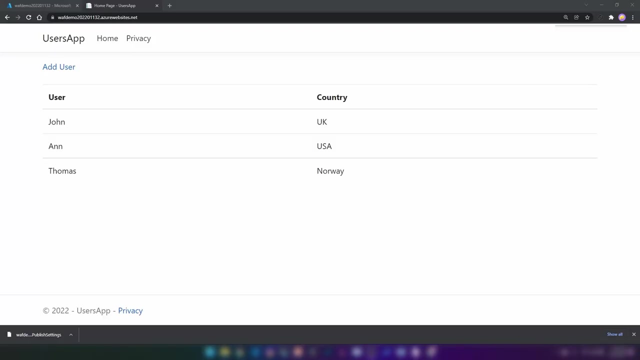 now let me go into Azure studio and here I have wrote a sample application. now let me add this published profile. all right, I'm going to click publish. as you can see, it is getting published now. all right, the application is up and running now. it is a simple application where we have a list of users and if I click here, 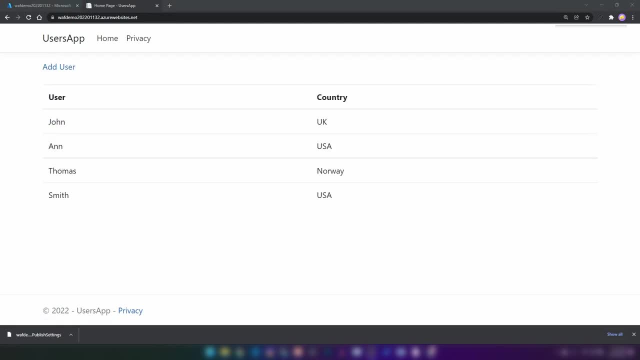 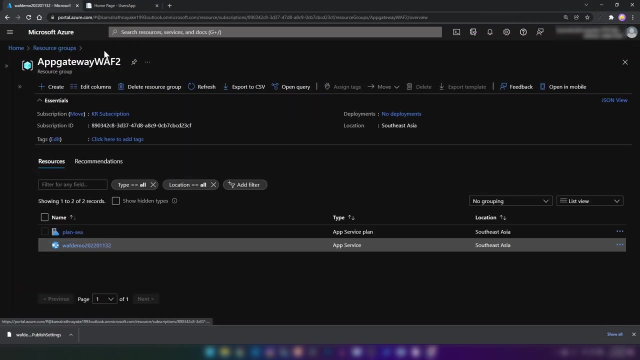 I do add the user. I can add a new user. now that we have our sample application in place, it is time for us to create the application gateway and start to understand how web application firewall works. now let me go back into Azure portal and I'm going into the resource group and I'm going to click create here. 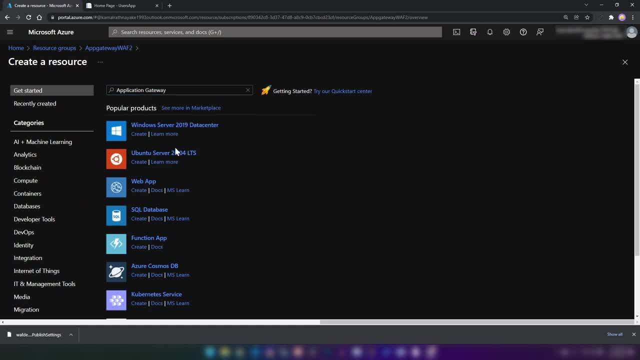 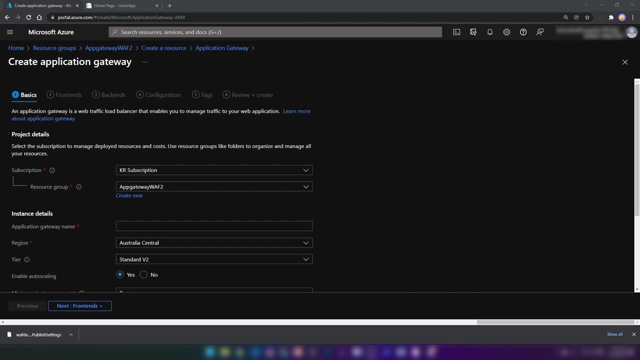 and then I'm going to search for application gateway. I'm going to click create here. if you also learn more about application Gateways and how to configure them, you can go ahead and watch my previous videos. I will link them down below in the description. now let me configure. 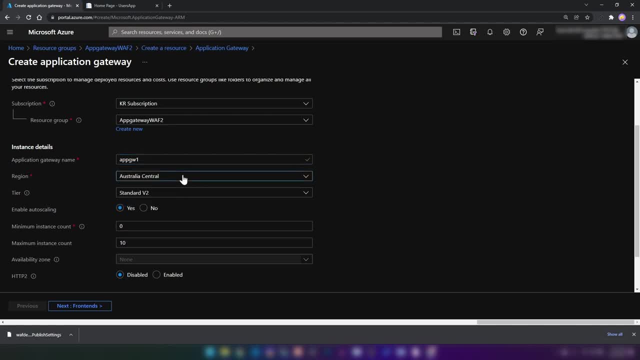 this for name. I'm going to call it app gateway. one region I want to go with: Southeast Asia. now we have to select the pricing tier. as you can see, we have standard and waaf tiers. you can go with standard tiers if you don't want web. 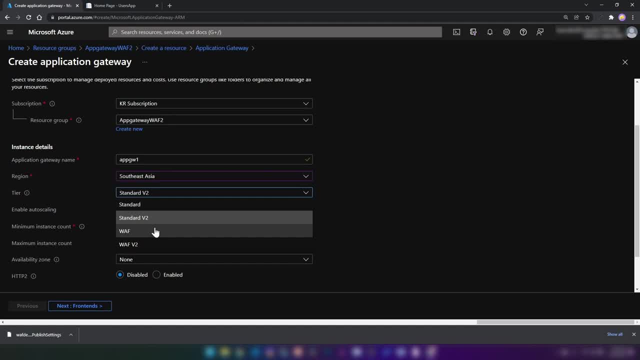 application firewall features. since i am going to talk about web application firewall in this video, i'm going with this tier, and also you can change this later as well. now what about this v2? this is a tier that has more features, such as auto scaling, zone redundancy and header rewrites, and faster. 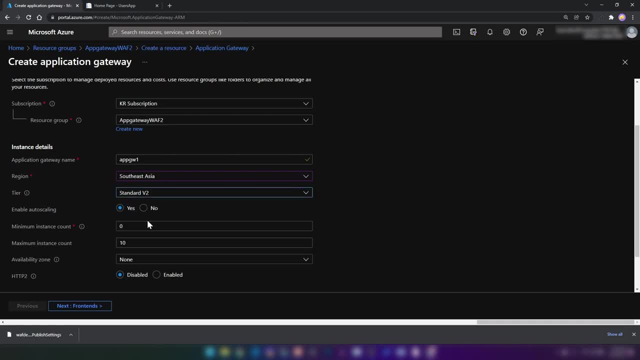 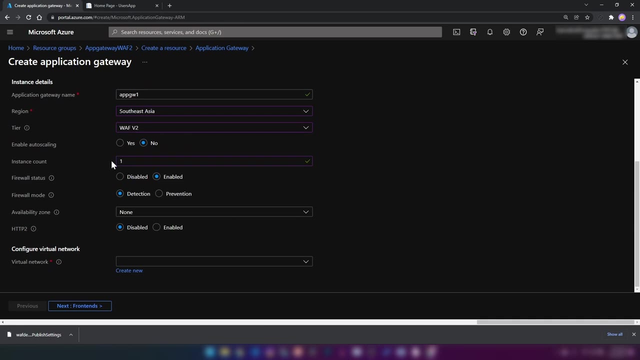 processing and improved performance and things like that. now, if i go with v2 tiers, as you can see, the auto scaling features gets enabled. i'm going with wav v2 tier for this video and i don't want to enable auto scaling, and one instance is okay for me and the firewall status is enabled. 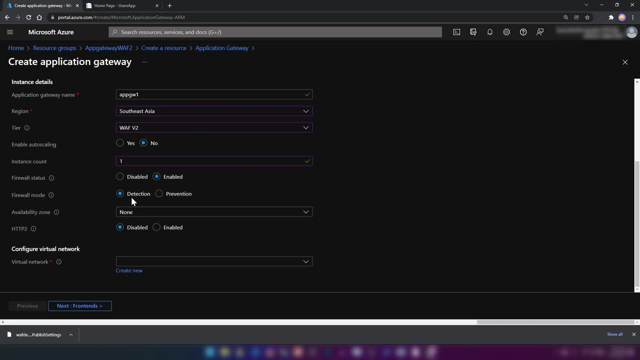 this is a important setting. what we tell application gateway here is that whether we need detection or prevention for malicious requests, as i said earlier, if i select this option, application gateway will detect the malicious request and it will lock them, but it will allow the request to travel to reach to our backends. but 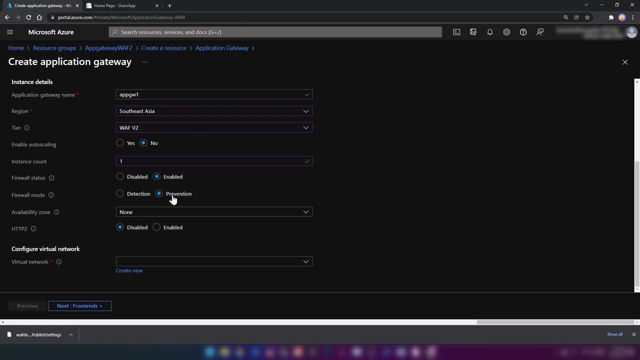 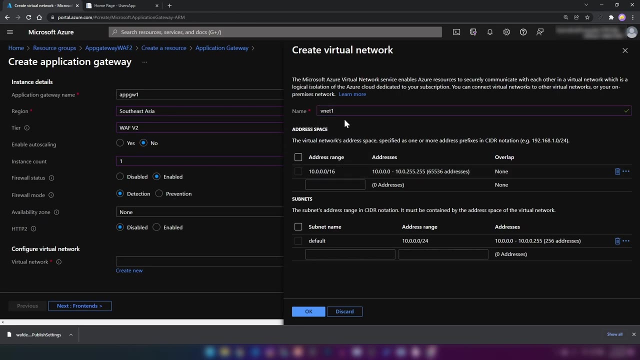 if i select this option here, the malicious user gets a 403 http response. i'm going to keep this one for now and then i'm not going to do any changes here. since we need a virtual network, let me create one now. i'm going to call it vnet1 and this address range and this address range for. 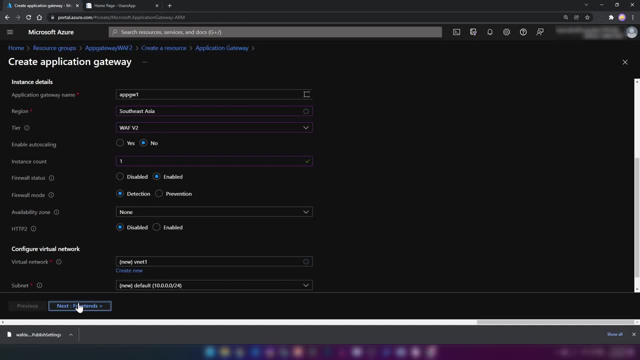 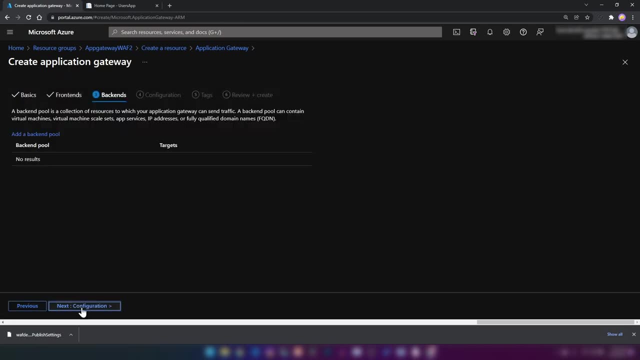 vnet is okay for me. and then i'm going ahead to create a public ip address, since we are accessing it from the public internet, and i'm going to add a backend pool- let me call it bp1- and then i'm going to select the app service that 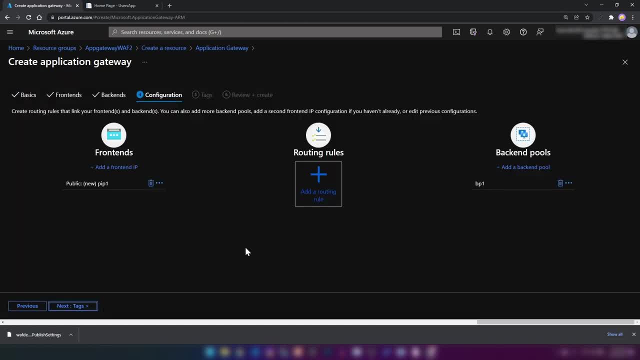 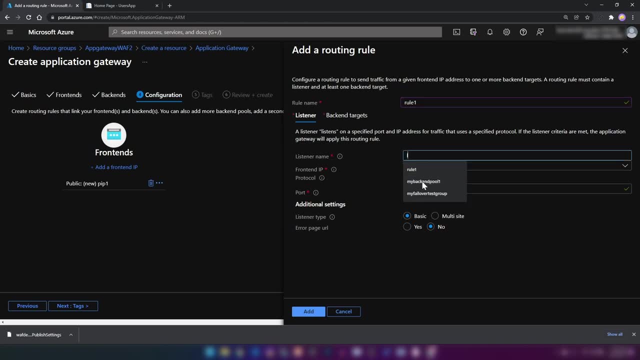 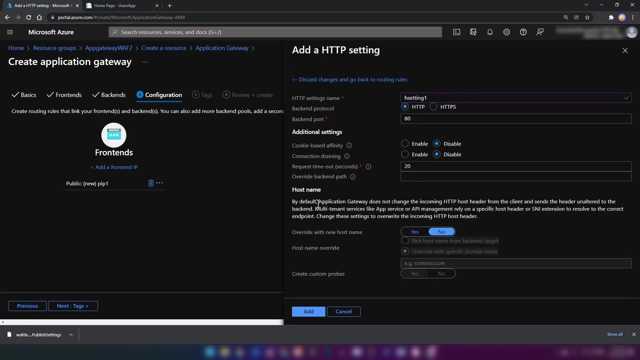 we have created. let me add that one. and then we need to add a routing rule. i'm going to go with rule one here, and we have to create a list as well. now, since we are integrating with an app service, we need to enable this feature to forward. 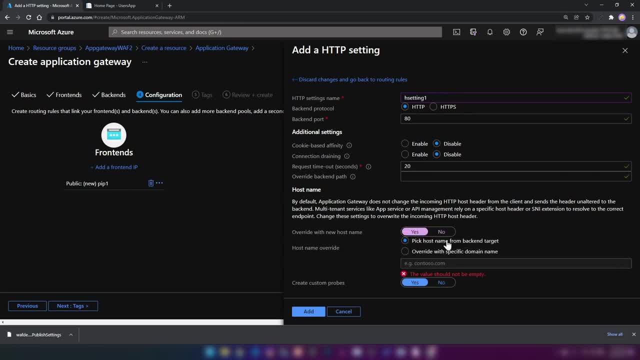 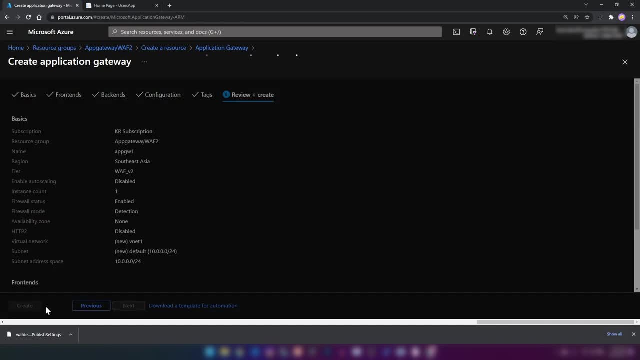 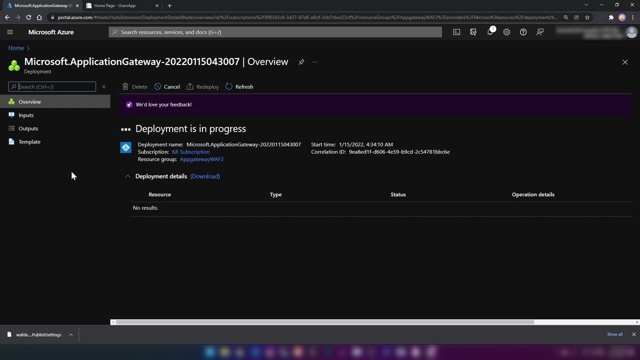 the host header. i'm going to go with this option: pick host name from the backend target. all right, i'm going to add the routing rule. i'm going to click next to create the application gateway. as you can see, it is getting deployed now. let's wait for around 10 minutes until this gets. 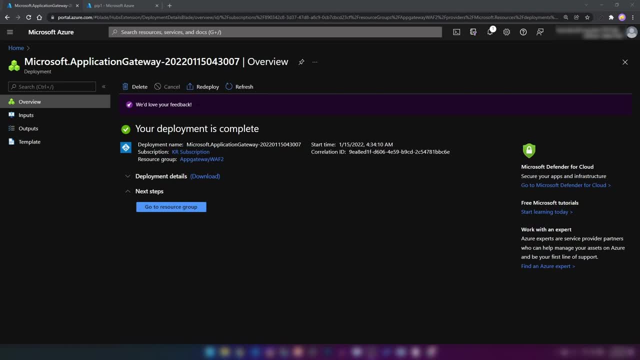 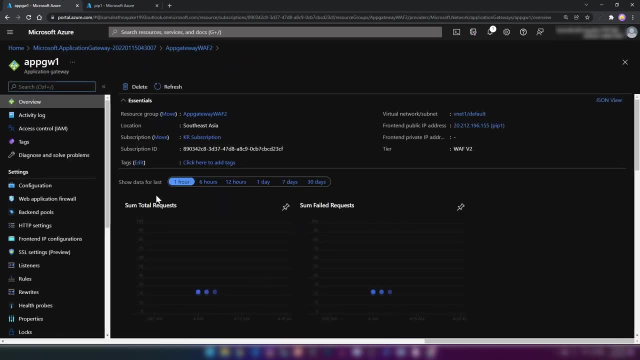 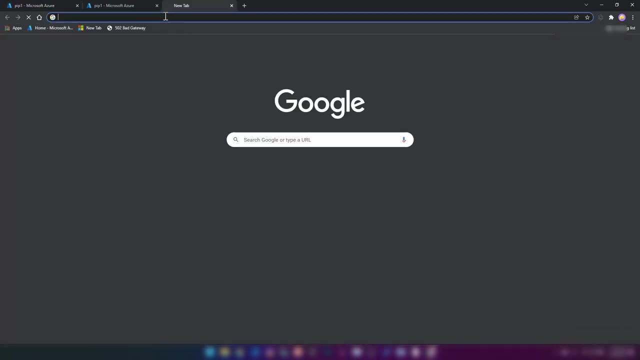 deployed. all right, as you can see, our application gateway instance is in place. now let me go to the resource group and then click on app gateway one. we have a public ip address here. let me click on it and i'm going to copy the public ip address and then i'm going to paste and go. as you can see, 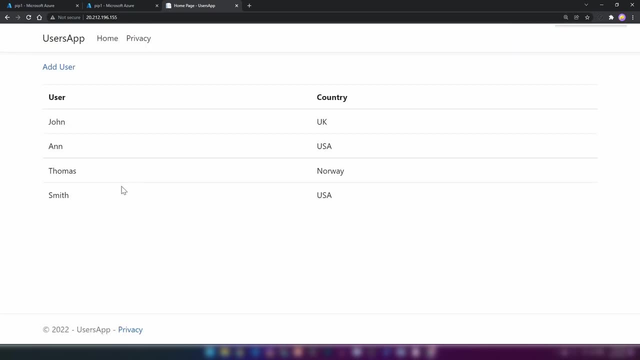 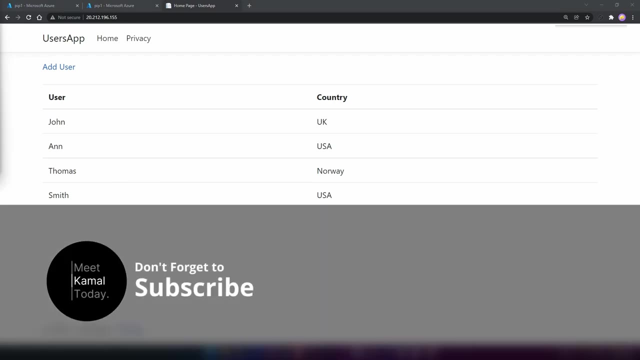 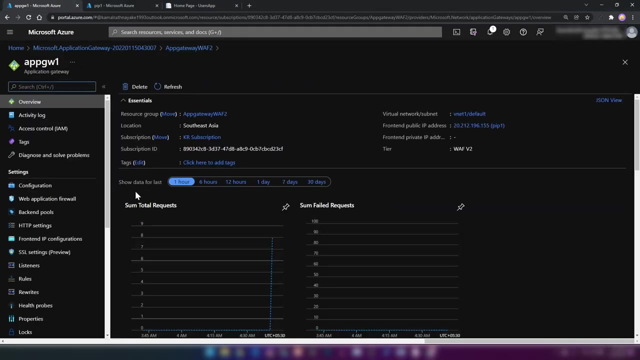 we can access our application with the public ip address of our application gateway, and now it's time for us to understand how web application firewall works. now, if i go back to the resource group and the application gateway, we have a tab here, web application firewall- in there as. 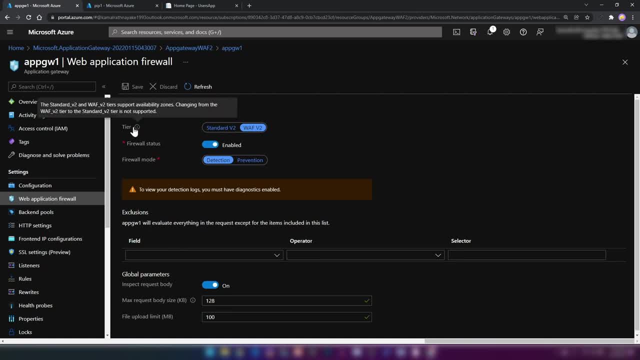 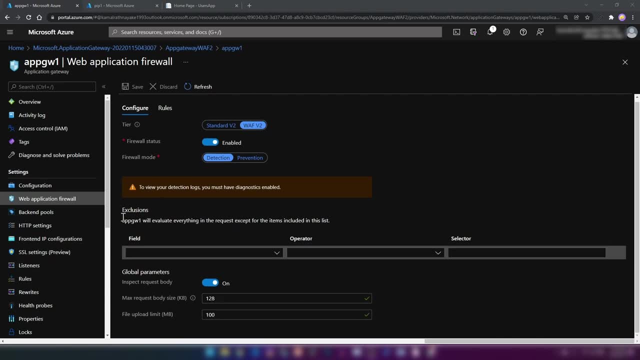 you can see, we can change the tier and also firewall status and these two modes as well. as you can see over here, we can add exclusions, we can add request headers, cookies and attributes and we can apply a operator and we can add some text here. we can add exclusions to the firewall. 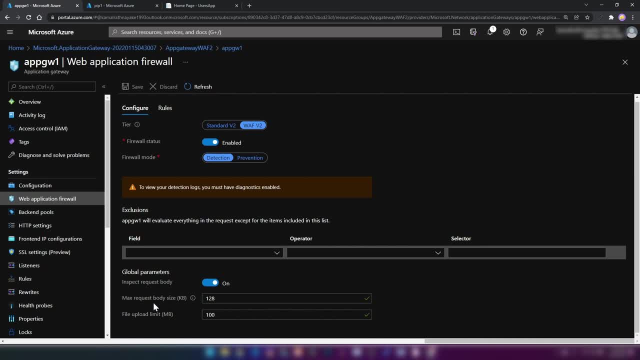 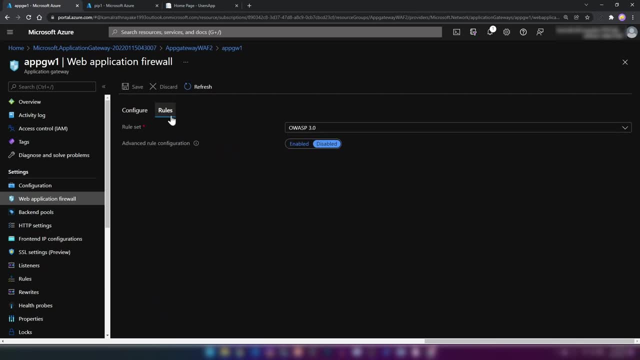 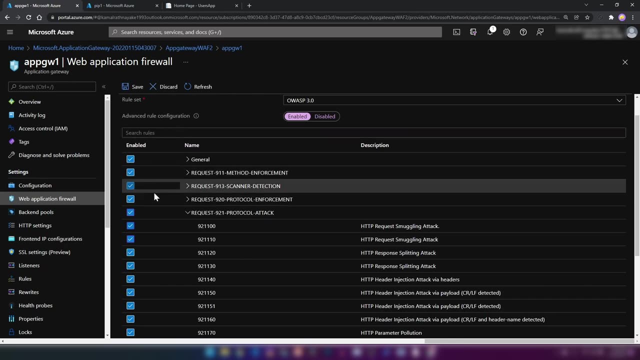 and also we can specify the max request body size and file upload limit as well. now, if i go into the rules, as you can see, we can specify the rule set. the default one here, as you can see, is three and if you want to enable or disable, basically modify this rule set, you can do it here like this: 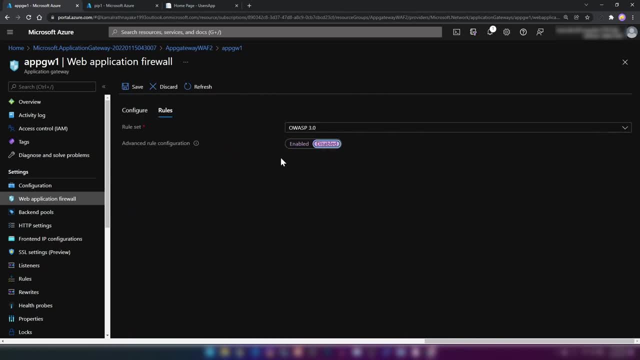 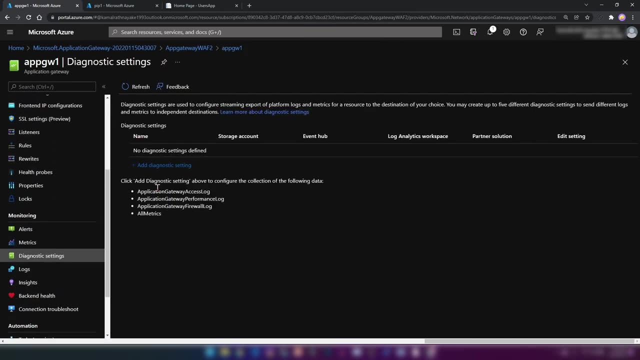 now i'm going to disable this advanced rule configuration here. i haven't done any changes here and if i go into diagnostic settings, we can attach a storage account or a log analytics workspace to log the events of this web application firewall. now let me add a diagnostic. i'm going to 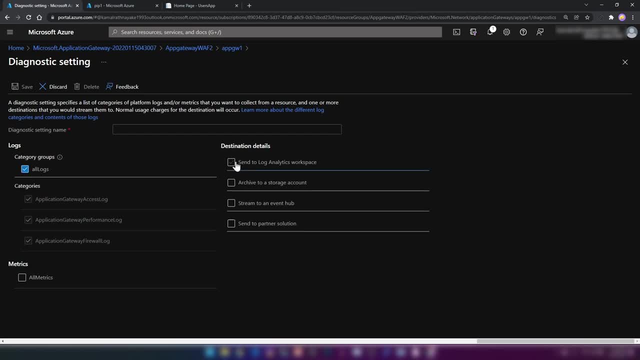 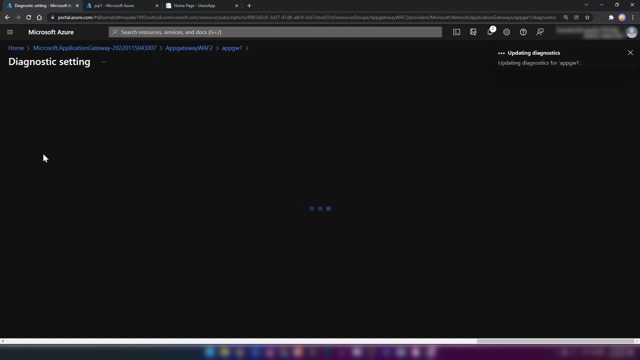 go with all logs, and then i'm going to select this option- send to log analytics workspace- and then i'm going to say log analytics workspace and then i'm going to select log analytics and then we're going to enable as well, and then i'm going to keep this setting my default log analytics workspace. 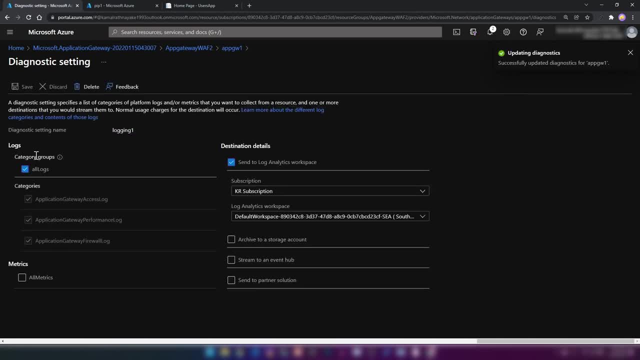 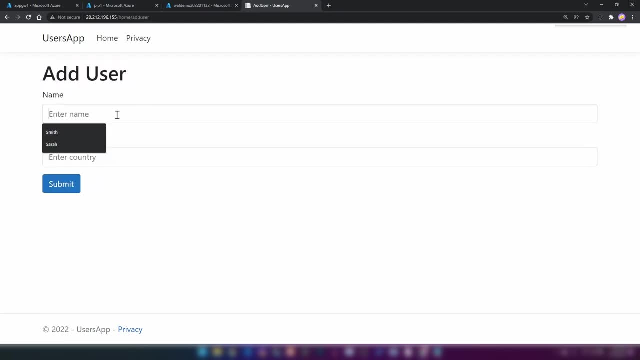 let me provide a name as well, and then i'm going to save this diagnostic setting so that we can see what happened in my application gateway. now i'm going into the app that we have deployed, and then i'm going to add a new user here. i'm going to select sara, and that is something that i've already. 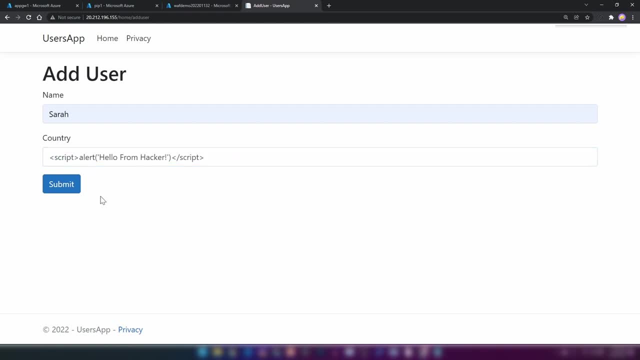 tried. let's see what happens. as you can see, the script that I have inserted got saved in the database. when I load the home page, I can see this message. I'm going to click OK and, as you can see, this app is vulnerable to attacks. I'm 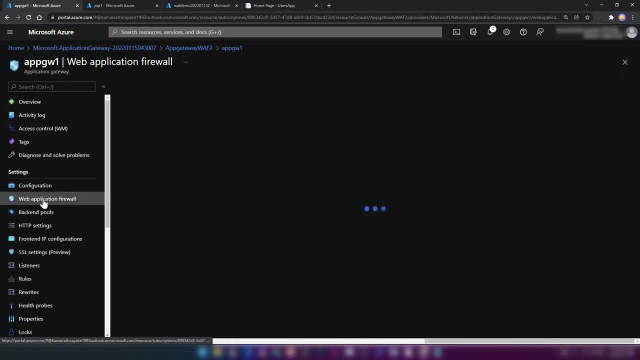 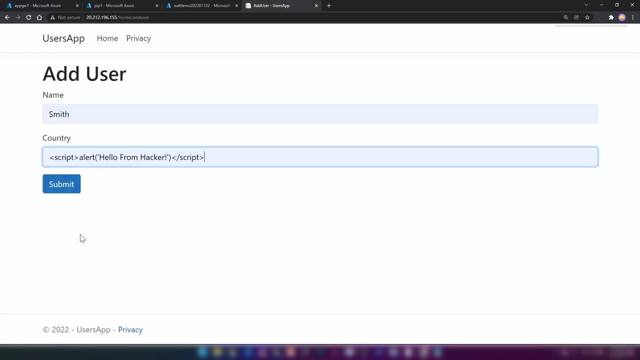 going into my Azure portal now and then I'm going to web application firewall and then I'm going to change this firewall mode from detection to prevention. let's see what happens now. I'm gonna save this one all right. now let me go back and user, and then I'm going to add the same script here. let me. 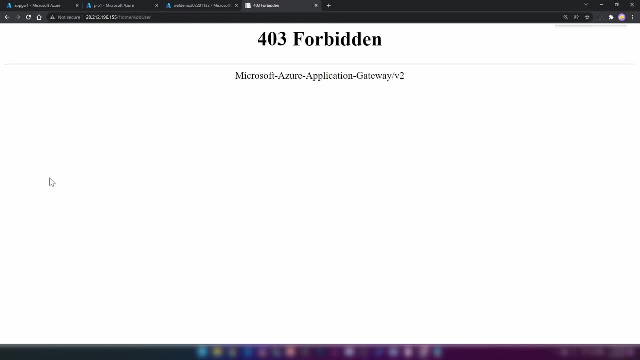 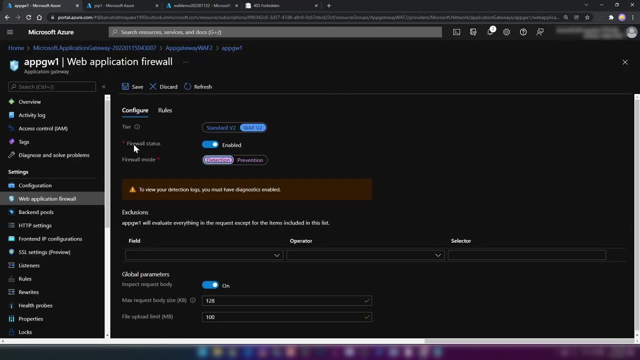 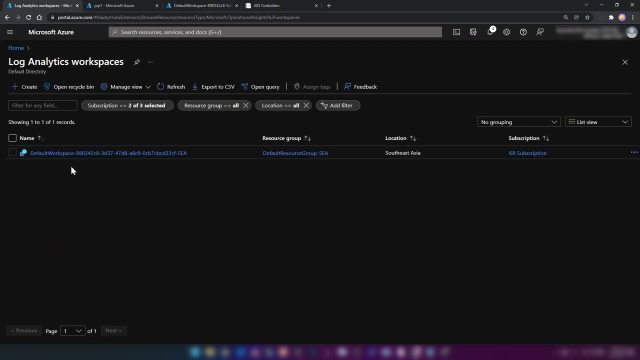 click Submit, as you can see now, as your application gateway blocks my request because it was a malicious one. now let me go back and change this back to detection mode. now, if I go into the log analytics workspace that I have configured, I'm going to select this one here. 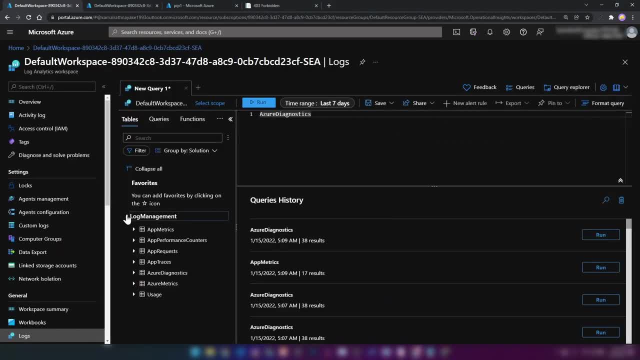 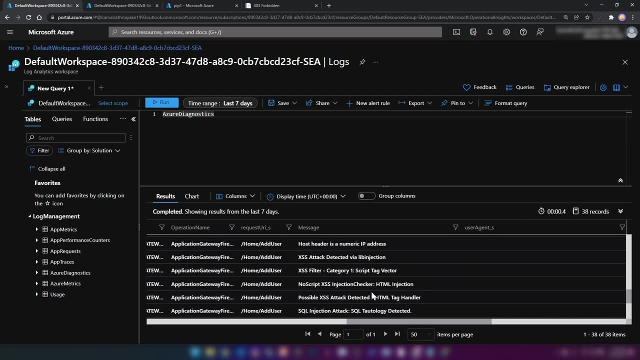 and let me close this and I'm going to query Azure Diagnostics- and, as you can see here, if you look at the message field and as you can see here, our web application firewall that we have configured has locked information about an SSS attack and this is how Azure application gateway web application. 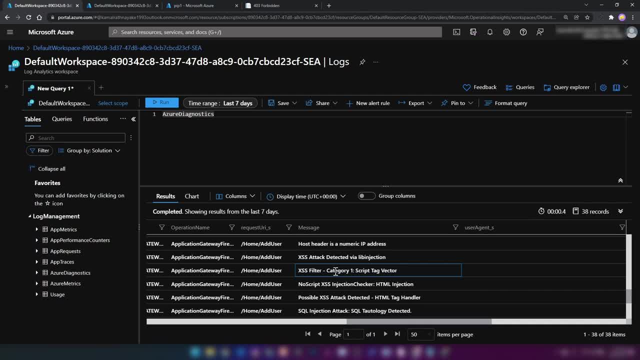 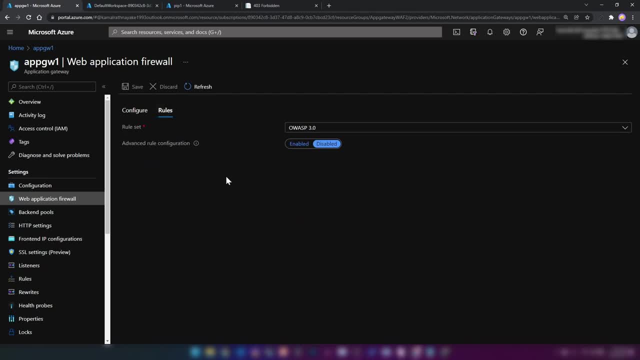 firewall helps you protect your web applications. now, if I go back to the application gateway, and I can see that the web application firewall is now in the application gateway and the web application firewall- the rules that we have here. these rules- they were defined by Azure. based on these, OWASP identified.